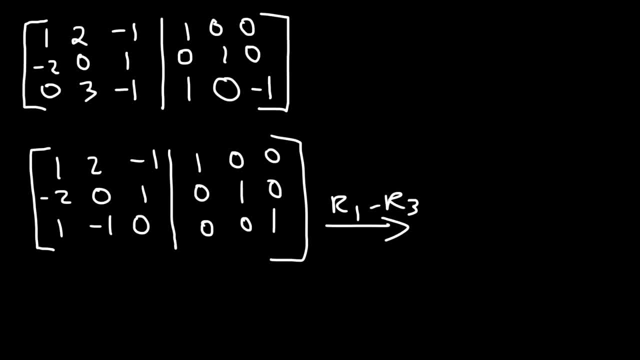 So that's negative 1.. So now, what do you think we need to do next? How can we turn this negative 2 into a 0? What row operations do we need to apply to row 2 to do so? So we're going to say 2 times R1 plus R2.. 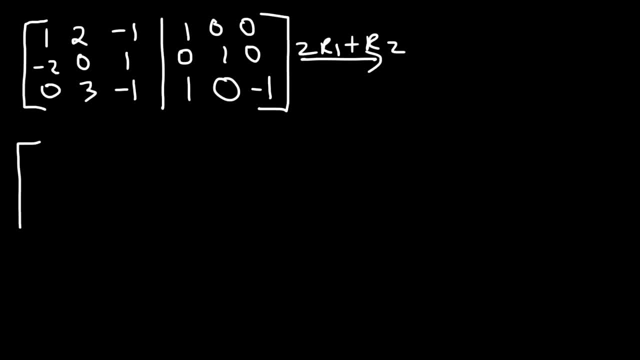 Let's do that. So we're changing row 2.. Row 1 is going to stay the same. Row 3 will remain the same as well. So 2 times 1 plus negative 2, that's going to be 0.. 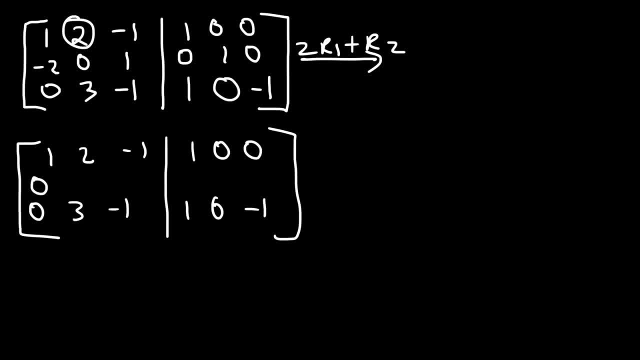 2 times 2 plus 0, that's going to be 4.. 2 times negative 1, which is negative. 2 plus 1, that's negative 1.. 2 times 1 plus 0 is going to be 2.. 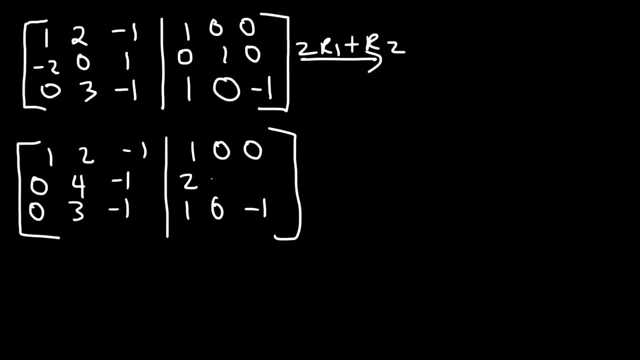 2 times 0 plus 1 plus 1, that's 1.. 2 times 0 plus 0 is 0.. Now let's turn that number into a 0.. So we need to apply the row operation to row 3.. 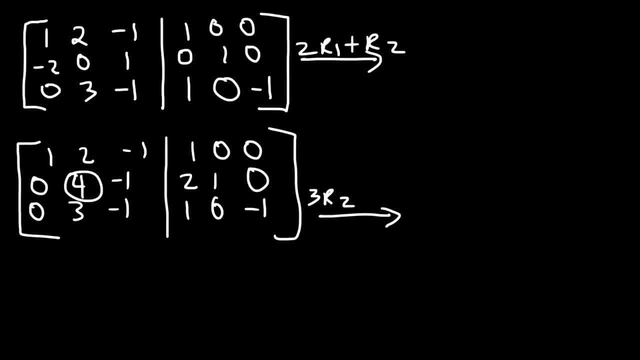 I'm going to multiply R2 by 3, because 3 times 4 is 12.. And then I'm going to multiply R3 by 3, because 3 times 4 is 12.. We're going to subtract it by 4 times R3, because negative 4 times 3 is negative 12, and they'll 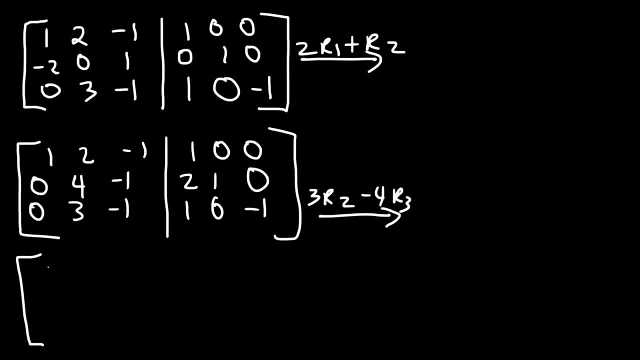 cancel to 0.. So row 1 is going to stay the same and let's rewrite row 2.. So we're going to have 3 times 0 minus 4 times 0, which is 0, and then 3 times 4 minus 4. 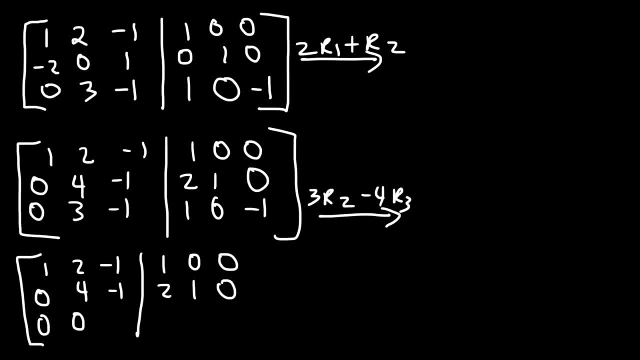 times 3, that's going to be 0 as well, And then 3 times negative 1, which is negative 3, minus 4 times negative 1, so we have negative 3 plus 4, that's going to equal to 1.. 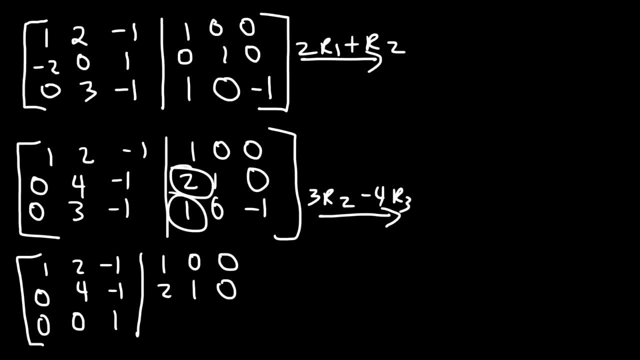 And then 3 times 2 is 6, minus 4 times 1, so 6 minus 4 is 2.. 3 times 1 minus 4 times 0, that's 3.. And 3 times 0 minus 4 times 1.. 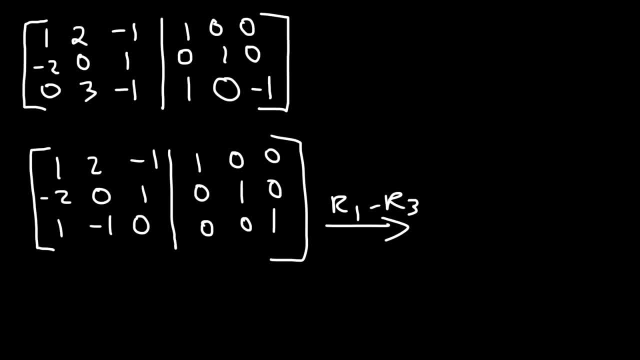 And then it's negative 1.. So now, what do you think we need to do next? How can we turn this negative 2 into a 0? What row operations do we need to apply to row 2 to do so? So we're going to say 2 times R1 plus R2.. 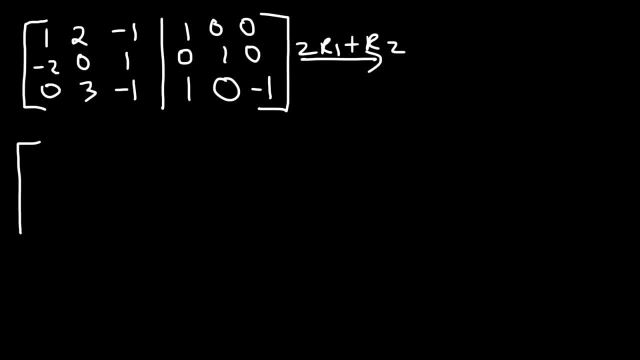 Let's do that, So we're going to say 2 times R1 plus R2.. Let's do that, So we're changing row 2.. Row 1 is going to stay the same. Row 3 will remain the same as well. 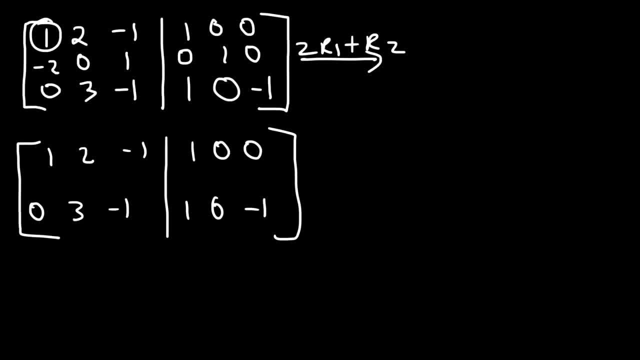 So 2 times 1, plus negative 2,, that's going to be 0.. 2 times 2 plus 0,, that's going to be 4.. 2 times negative 1, which is negative, 2 plus 1.. 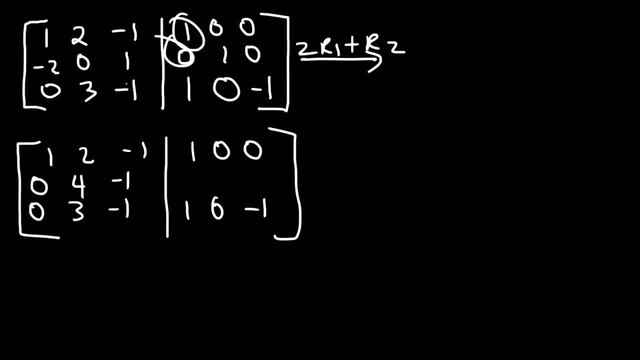 negative: 1.. 2 times 1 plus 0 is going to be 2.. 2 times 0 plus 1, that's 1.. 2 times 0 plus 0 is 0.. Now let's turn that number into a 0.. So we need to apply the row operation to row 3.. 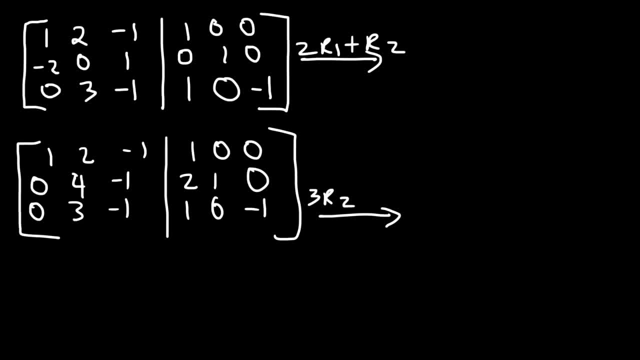 I'm going to multiply R2 by 3, because 3 times 4 is 12.. And then I'm going to subtract it by 4 times R3, because negative 4 times 3 is negative 12. And they'll cancel to 0.. 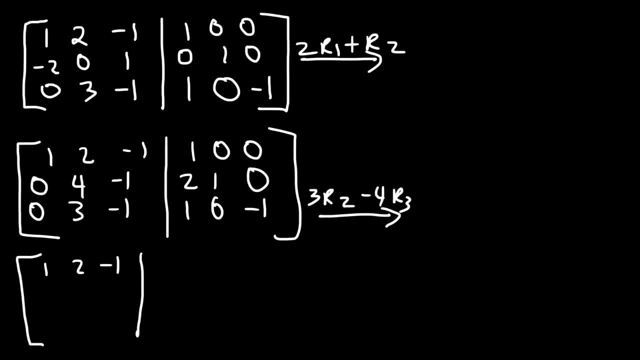 So row 1 is going to stay the same And let's rewrite row 2.. So we're going to have 3 times 0 minus 4 times 0, which is 0.. And then 3 times 4 minus 4 times 3,. 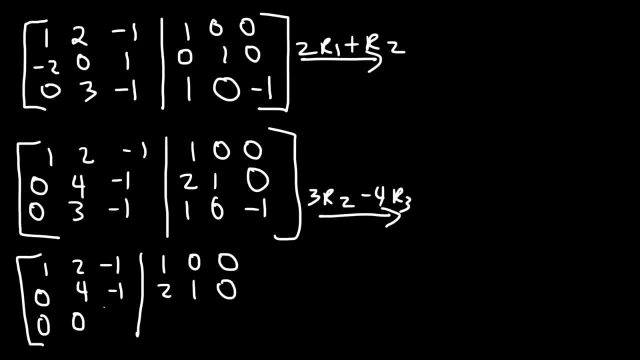 that's going to be 0 as well. And then 3 times 4 minus 4,, which is 0.. 3 times 0 minus 4 times 3,, which is 0.. And then 3 times 4 minus 4 times 3,, that's going to be 0 as well. 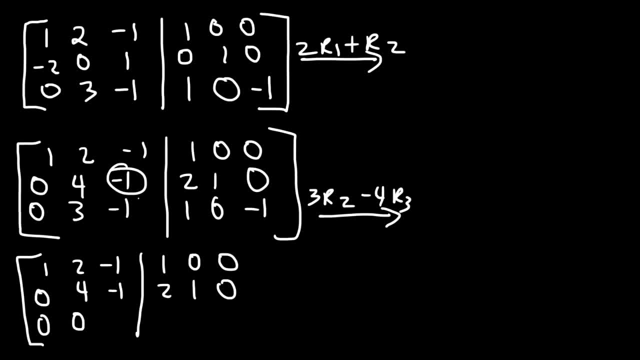 negative 1, which is negative 3 minus 4 times negative 1. so we have negative 3 plus 4. that's going to equal to 1, and then 3 times 2 is 6 minus 4 times 1. so 6 minus 4 is 2, 3 times 1 minus 4 times 0, that's 3 and 3 times 0 minus 4 times. 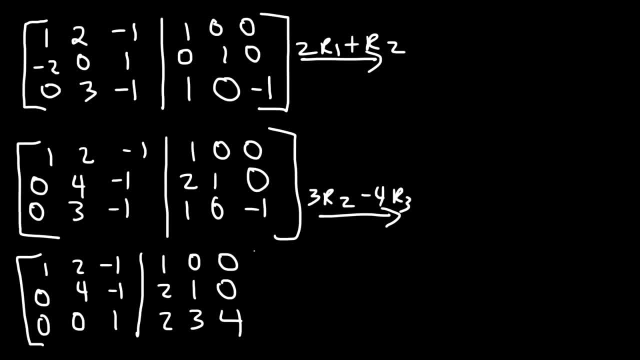 3 times negative, 1 is 4.. Now what we need to do is turn this number into a 0.. So that's going to be straightforward. We just got to add row 1 and row 3 to accomplish that. So let's rewrite rows 2 and 3.. 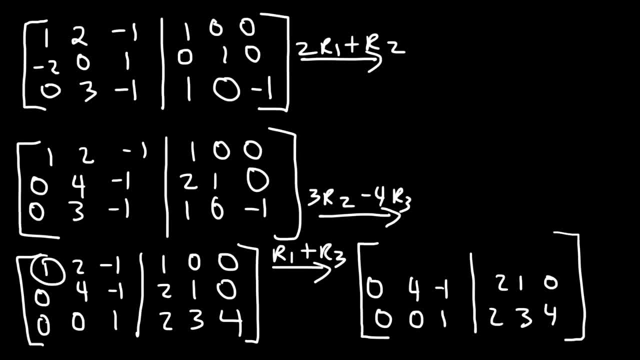 So it's going to be 1 plus 0, which is 1.. And then 2 plus 0, that's 2.. Negative 1 plus 1 is 0. And then 1 plus 2 is 3.. 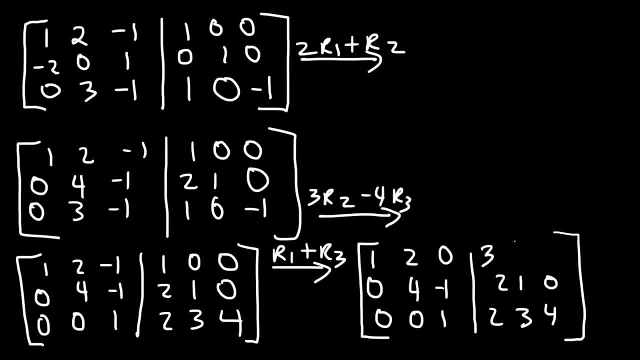 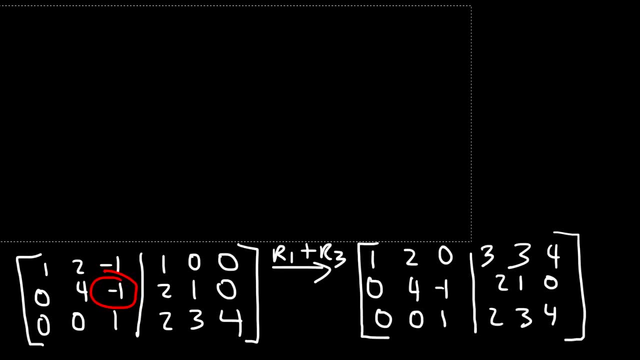 And then 0 plus 3 is 3.. Alright, 0 plus 4 is 4.. Now let's focus on that number. What row operations do we need to apply to row 2 in order to make it 0?? All we need to do here now is add row 2 and 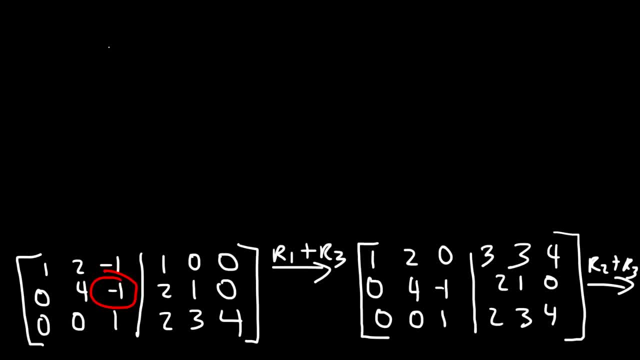 row 3.. So notice what's going to happen. So let's rewrite row 1.. Now let's rewrite row 3.. So row 2 plus row 3, 0 plus 0 is 0. And then 4 plus 0 is 4.. Negative: 1 plus 1,. 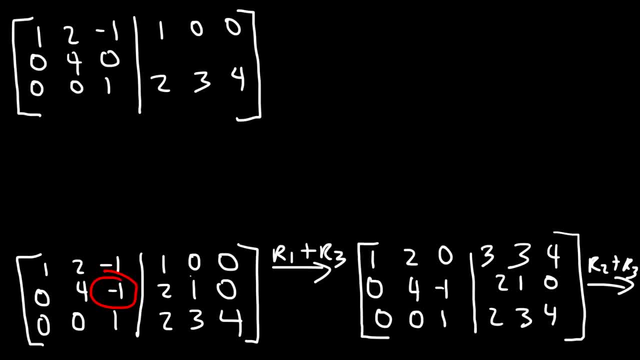 that's going to be 0. And then we have 2 plus 2,, which is 4.. And 1 plus 3,, that's 4.. and then 0 plus 4 is also 4.. Now what we need to do at this point? wait, hold on. I didn't copy this. 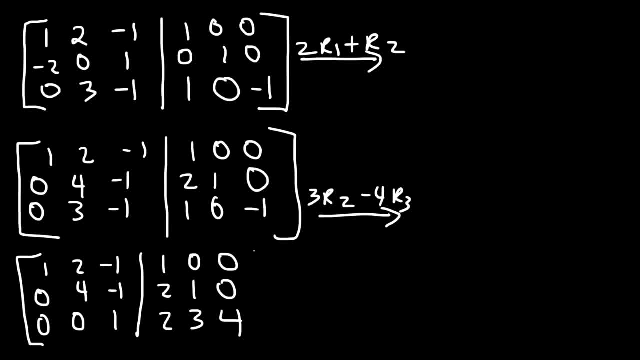 negative 1 is 4. now what we need to do is turn this number into a 0, so that's going to be straightforward: we just got to add the row 1 and row 3 to accomplish that, so let's rewrite rows 2 and 3. 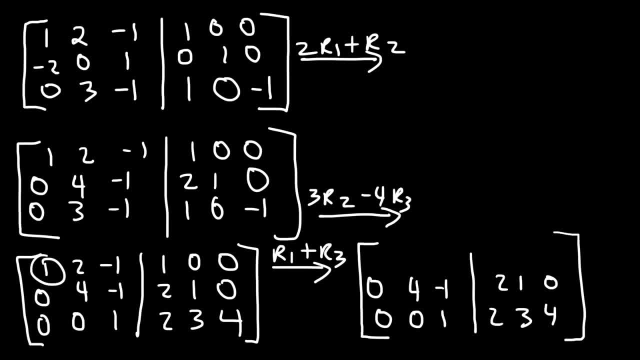 so it's going to be 1 plus 0, which is 1, and then 2 plus 0, that's 2 negative. 1 plus 1 is 0, and then 1 plus 2 is 3, and then 0 plus 3 is 3. 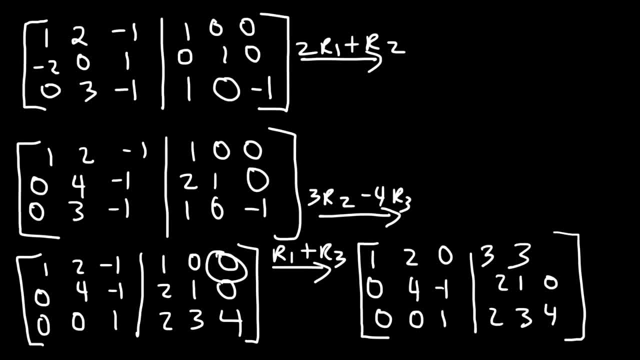 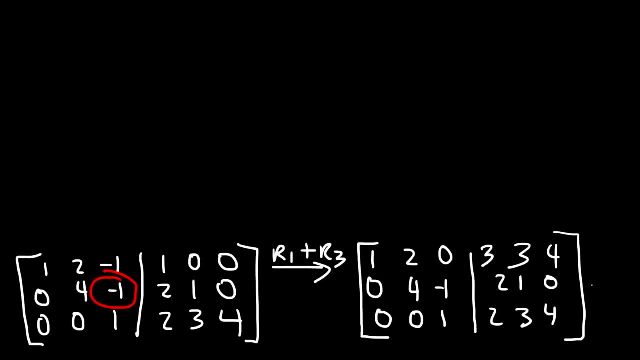 and 0 plus 4 is 4. now let's focus on that number. what row operations do we need to apply to row 2 in order to make it 0? all we need to do here now is add row 2 and row 3, so notice what's going to happen. so let's rewrite row 1. 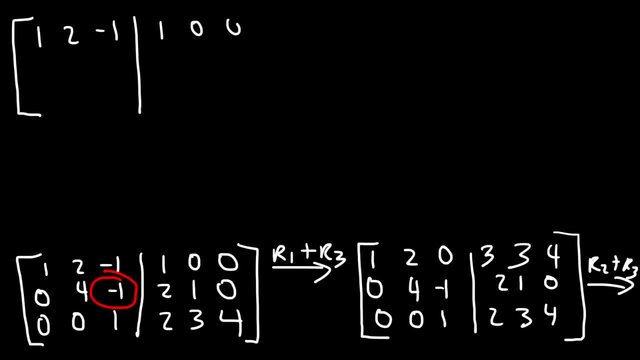 and let's rewrite Row three, so row 2 plus row 3, zero plus 0 is 0, and then 4 plus 0 is 4, negative. 1 plus 1, that's going to be 0, and then we have 2 plus 2, which is 4, and 1 plus 3. 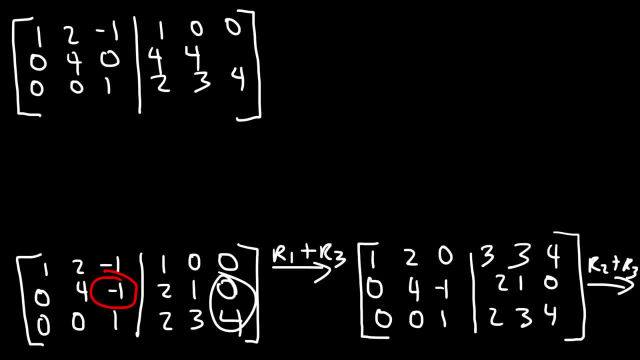 that's 4, And then 0 plus 4 is also 4.. Now what we need to do at this point? Wait, hold on. I didn't copy this correctly. This is supposed to be 1, 2, 0.. 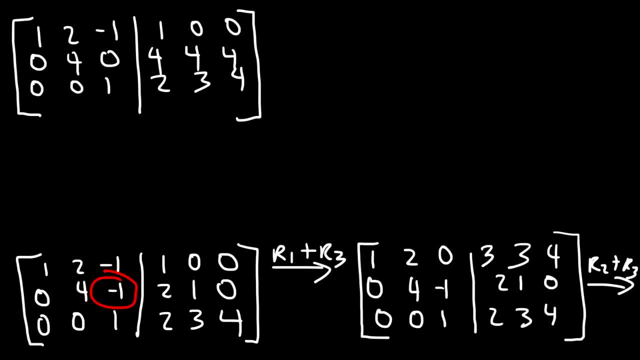 correctly, This is supposed to be 1,, 2, 0, and 3,, 3, 4.. So everything else should be fine at this point. This is what I should have right now. So at this point we need to turn this number into a 0.. So we need to apply the operation to row 1.. So let's take 2 times R1. 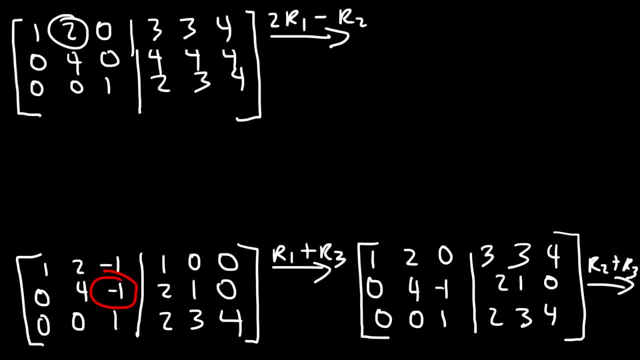 and subtract it by R2.. So we're going to have 0, 0,, 1,, 2,, 3,, 4, and then 0, 4,, 0,, 4,, 4, 4.. 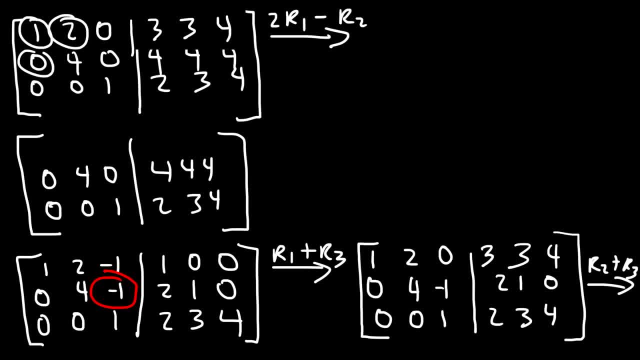 Now we're going to take 0, 0,, 1,, 2,, 3, 4, and then 0, 4, 0, 4, 4, 4.. 2 times 1 minus 0, so that's going to stay 1.. And then 2 times 2 minus 4, that is now 0.. 2 times 0 minus 0 is 0. 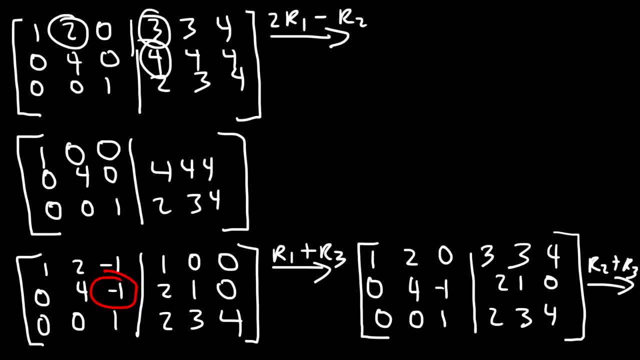 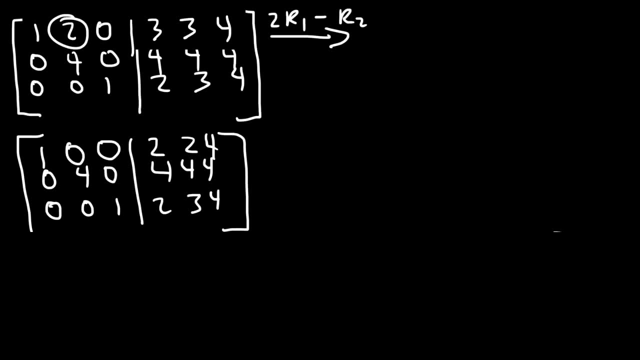 And then 2 times 3,, which is 6, minus 4, that's 2.. The next one is going to be the same: 2 times 4 is 8, minus 4 is 4.. And one thing I do need to fix: 2 times 1 minus 0,, that's supposed to be 2.. And I have a 1 here, so let's fix that. 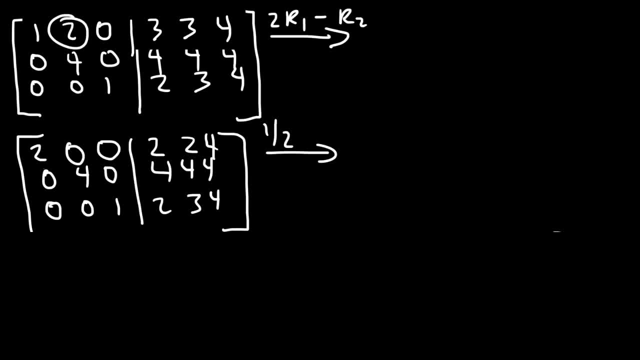 Now what we need to do is multiply the first row by 1 half and the second row by 1 over 4.. And that should give us what we need. So half of 2, is 1. And half of 4 is 2.. 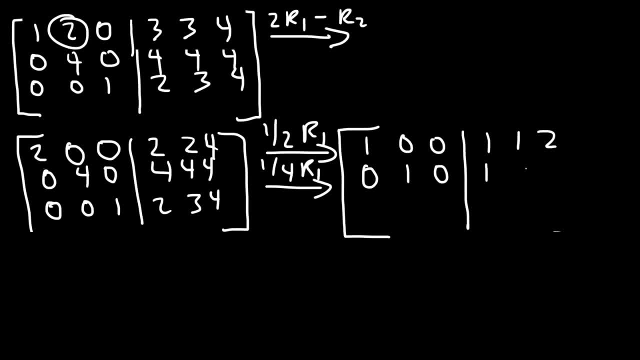 1 fourth of 4 is 1.. So all of these will be 1.. And then the last one is not going to change. So notice that here we have the multiplicative identity matrix I3.. And this side represents the inverse of matrix A. 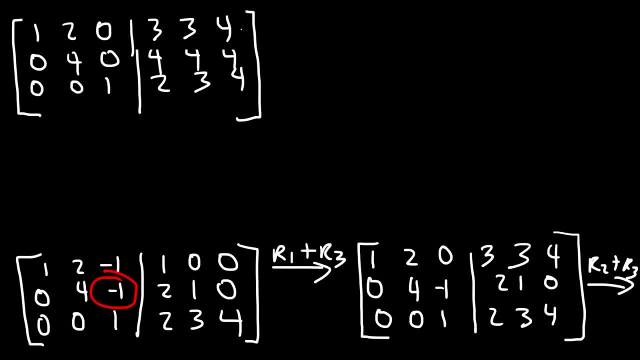 And 3,, 3,, 4.. So everything else should be fine at this point. This is what I should have right now. So at this point we need to turn this number into a 0.. So we need to apply the operation to row 1.. 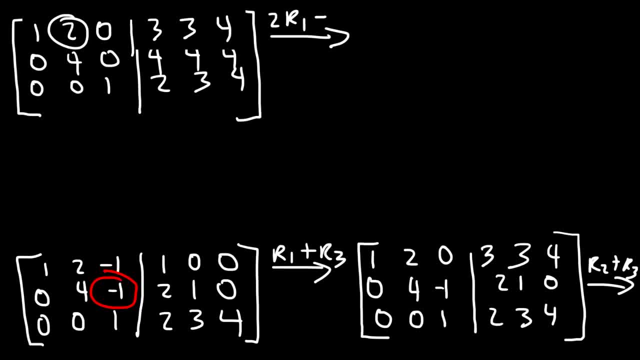 So let's take 2 times R1 and subtract it by R2.. So we're going to have 0, 0, 1,, 2,, 3,, 4, and then 0, 4, 0, 4,, 4, 4.. 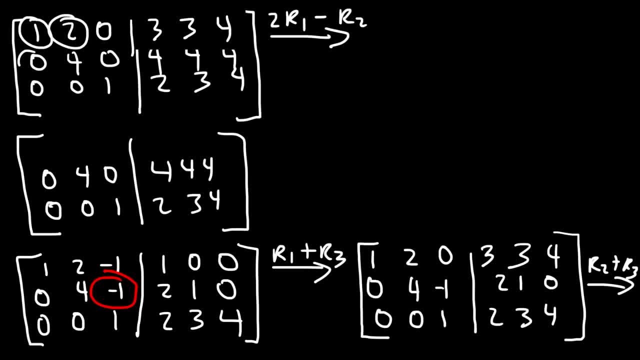 Now we're going to take 2 times 1 minus 0, so that's going to stay 1.. And then 2 times 2 minus 4, that is now 0.. So 2 times 0 minus 0 is 0.. 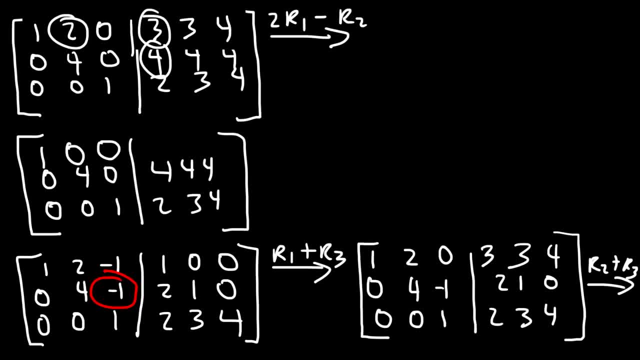 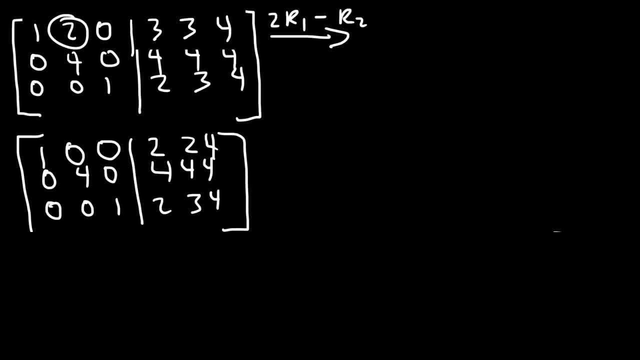 And then 2 times 3, which is 6, minus 4, that's 2.. The next one is going to be the same: 2 times 4 is 8, minus 4 is 4.. And one thing I do need to fix: 2 times 1 minus 0,, that's supposed to be 2.. 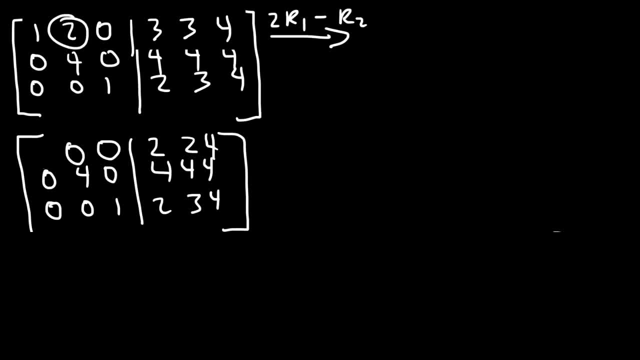 And I have a 1 here, So let's fix that. Now what we need to do is multiply the first row by 1 half And the second row by 1 over 4. And that should give us what we need. 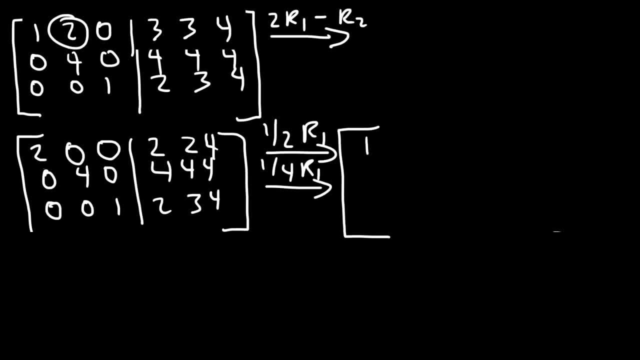 So half of 2 is 1. And half of 4 is 2.. 1 fourth of 4 is 1.. So all of these will be 1.. And then the last one is not going to change. So notice that here we have the multiplicative identity matrix I3.. 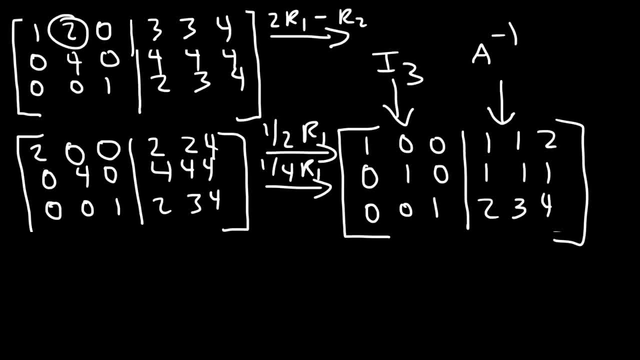 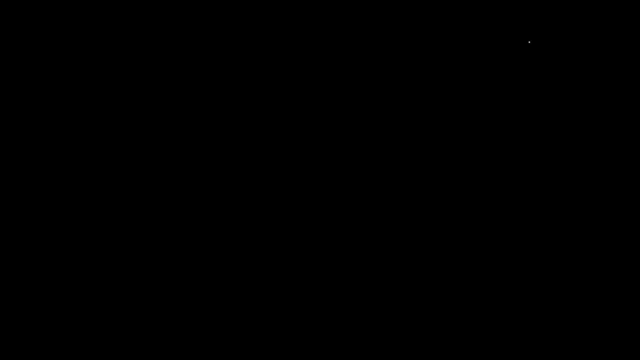 And this side represents the inverse of matrix A: 1, 1, 2, 1, 1, 1, 2, 3, 4.. Now, to confirm that it's indeed the inverse, what we need to do is multiply matrix A by 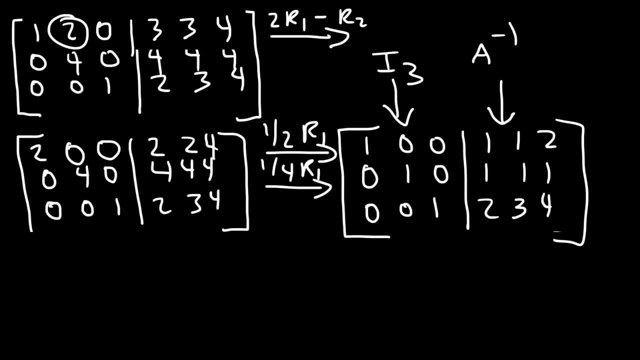 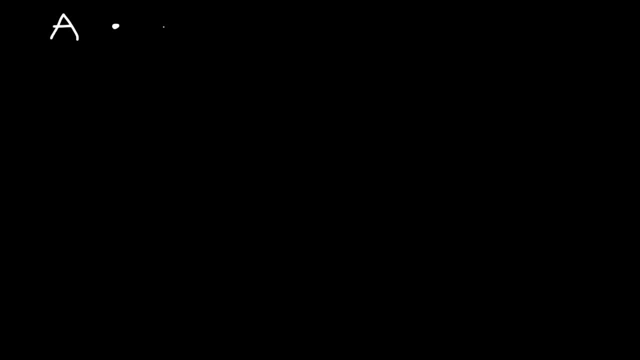 1, 1, 2.. 1, 1, 1, 2.. 3, 4.. Now to confirm that it's indeed the inverse, what we need to do is multiply matrix A by the inverse of A and show that it's equal to I3.. 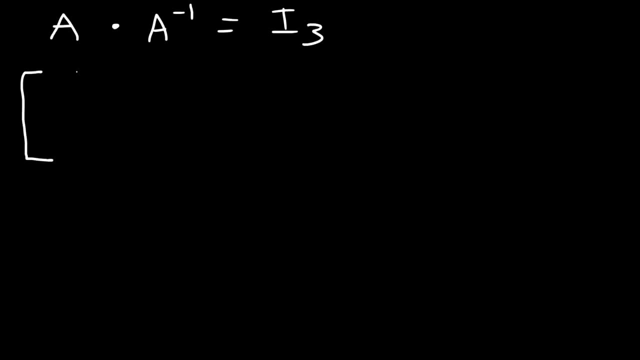 So, in other words, we need to take matrix A, which was 1, 2, negative, 1, negative, 2, 0, 1, 1, negative, 1, 0, and multiply it by the inverse of that matrix, which is 1.. 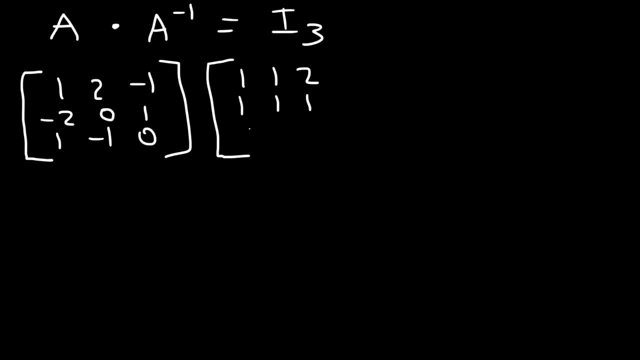 1, 1, 2.. 1, 1, 1, 2, 3, 4.. And if this is the matrix of A, if we did it correctly, we should get this answer: 1, 0, 0.. 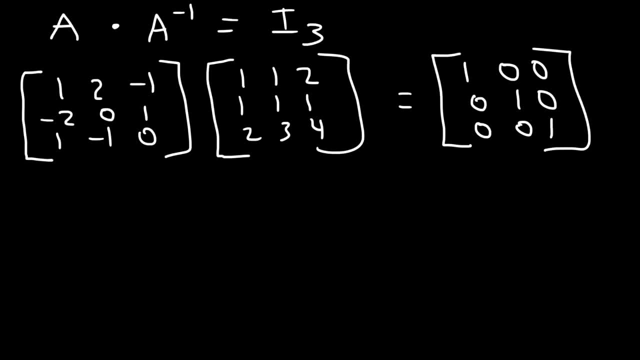 0, 1, 0.. 0, 0, 1.. So let's find out if we did it correctly. So I'm going to put my answers in here First. we need to take the first row and multiply it by the first column. 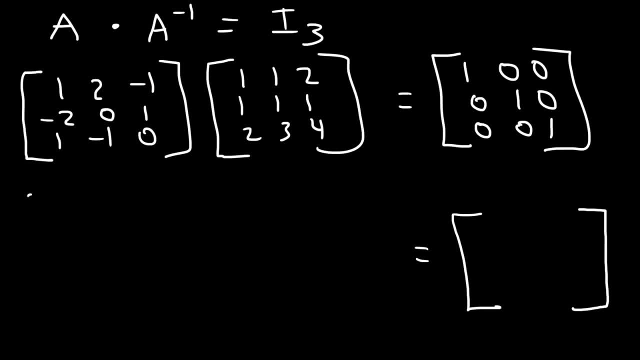 And add the products. So it's going to be 1 times 1.. So we're multiplying these two first, And then it's going to be plus 2 times 1.. That's these two, And then plus negative 1 times 2.. 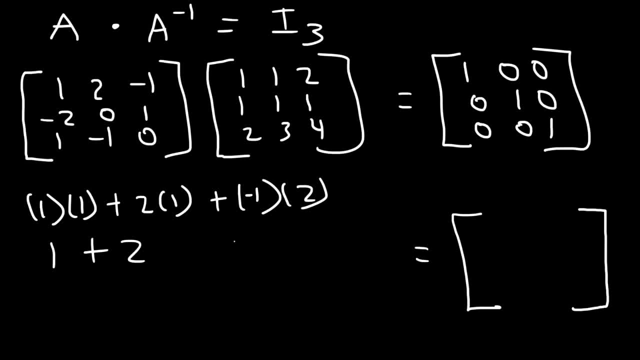 So 1 times 1 is 1.. 2 times 1 is 2.. Negative 1 times 2 is negative, 2.. These two cancel, and so we get 1.. So we have the first entry. Now let's multiply row 1 by column 2.. 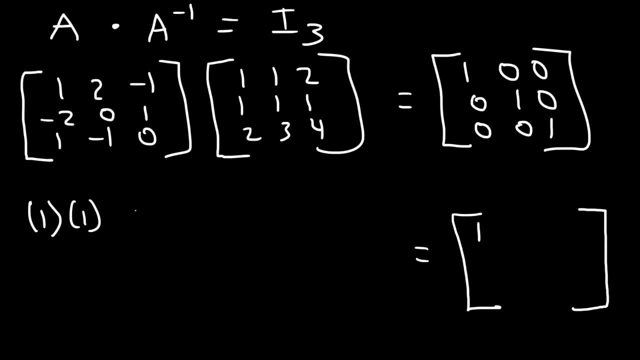 So it's going to be 1 times 1 plus 2 times 1 plus negative, 1 times 3.. So this is 1 plus 2 minus 3.. 1 plus 2 is 3.. 3 minus 3 is 3.. 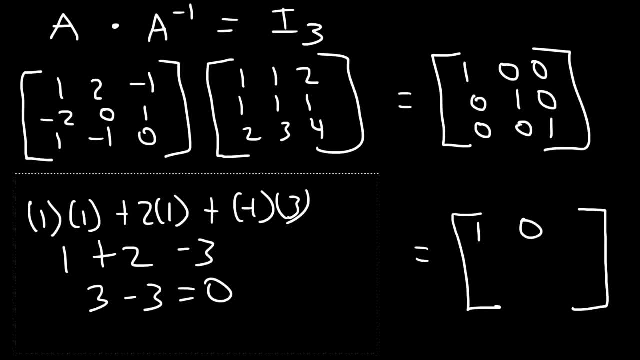 3 is 0.. Now let's try row 1 by column 3. So that's 1 times 2 plus 2 times 1, plus negative 1 times 4.. So this is 2, 2 minus 4.. 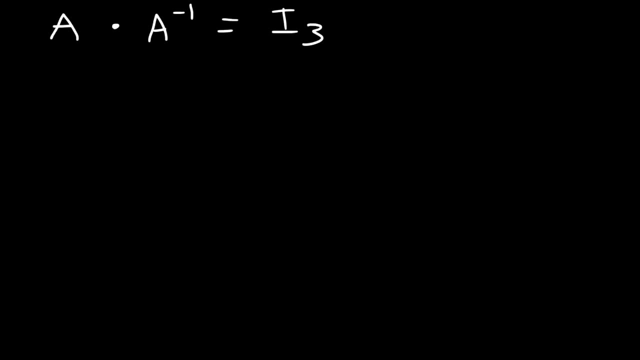 the inverse of A and show that it's equal to I3.. So we're going to do that. So, in other words, we need to take matrix A, which was 1, 2, negative, 1, negative, 2,. 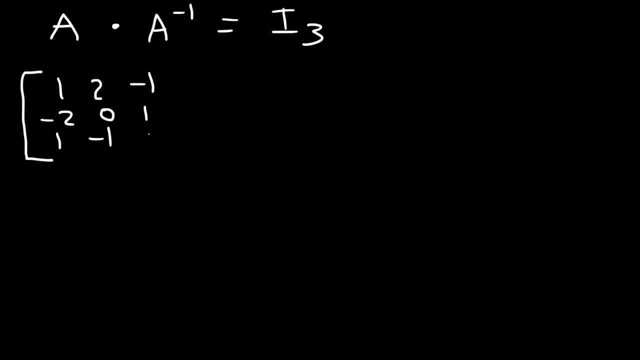 0, 1, 1, negative 1, 0.. And multiply it by the inverse of that matrix, which is 1, 1, 2, 1, 1, 1, 2, 3, 4.. 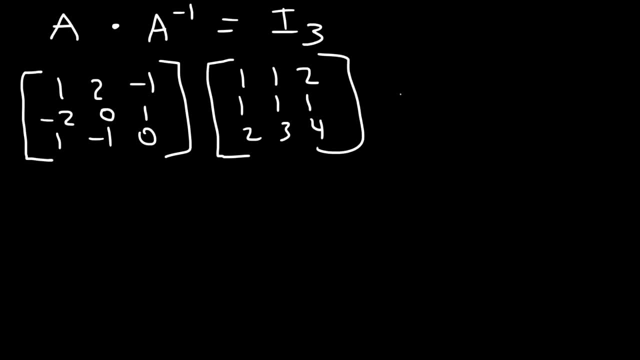 And if this is the matrix of A, if we did it correctly, we should get this answer: 1, 0, 0.. 0, 1, 0, 0, 0, 1.. So let's find out if we did it correctly. 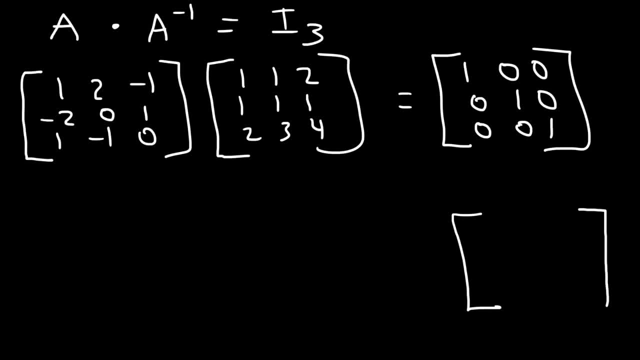 So I'm going to put my answers in here First. we need to take the first row and multiply it by the first column and add the products. So it's going to be 1 times 1.. So we're multiplying these two first. 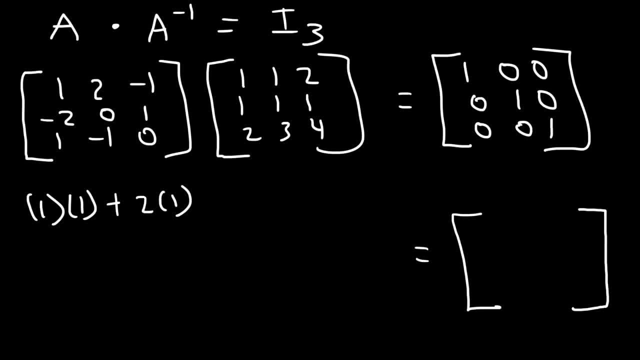 And then it's going to be plus 2 times 1.. these two and then plus negative 1 times 2. so 1 times 1 is 1, 2 times 1 is 2 negative. 1 times 2 is negative 2. these two cancel, and so we get 1. so we have. 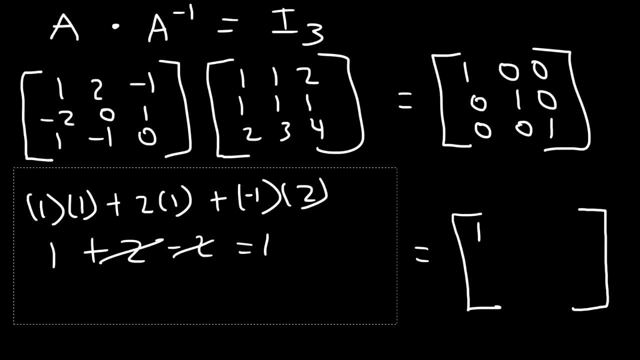 the first entry. now let's multiply row 1 by column 2, so it's going to be 1 times 1 plus 2 times 1, plus negative 1 times 3. so this is 1 plus 2 minus 3. 1 plus 2 is 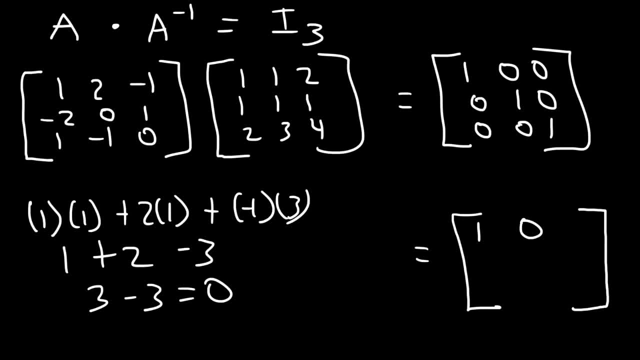 3, 3 minus 3 is 0. now let's try row 1 by column 3, so that's 1 times 2 plus 2 times 1, plus negative 1 times 4, so this is 2, 2 minus 4. 2 plus 2 is 4. 4 minus 4 is 0. 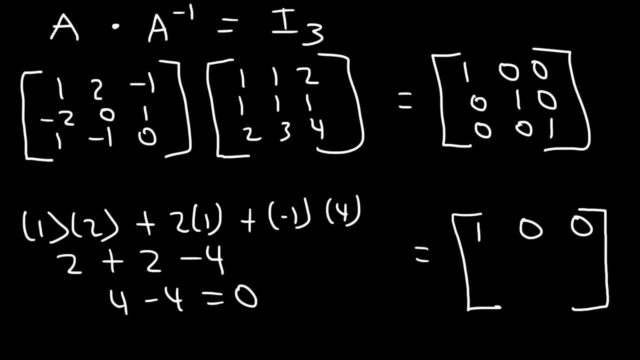 2 plus 2 is 4.. 4 minus 4 is 0.. Now let's move on to row 2.. Now let's multiply it by column 1.. So it's going to be negative 2 times 1 plus 0 times 1 plus 1 times 2.. 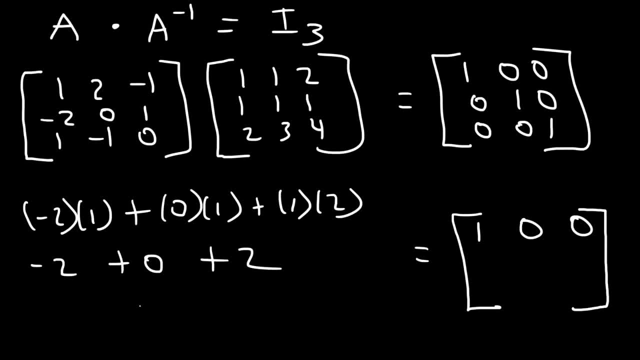 So this is negative 2 plus 0 plus 2.. Negative 2 plus 2 is 0.. Now let's take row 2 and multiply it by column 2.. So it's going to be negative 2 times 1 plus 0 times 1 plus 1 times 3.. 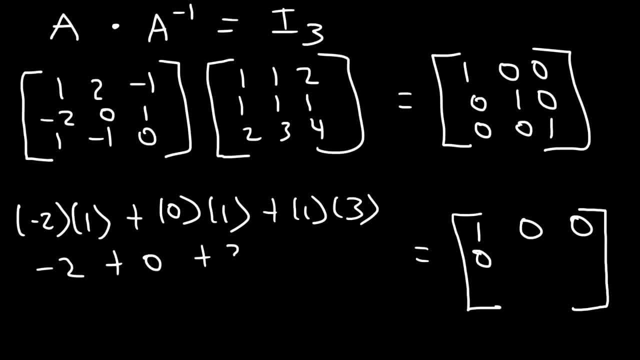 So that's negative 2 plus 0 plus 3.. Negative 2 plus 3 is 1.. Now let's multiply row 2 by column 3.. So negative 2 times 2 plus 0 times 1 plus 1 times 4.. 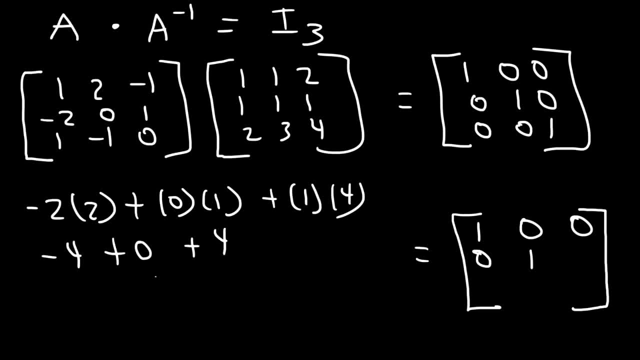 So this is going to be negative 4 plus 0 plus 4, which adds up to 0.. Now row 3 times column 1.. Let's try that. So it's going to be 1 times 1 plus negative, 1 times 1 plus 0 times 2.. 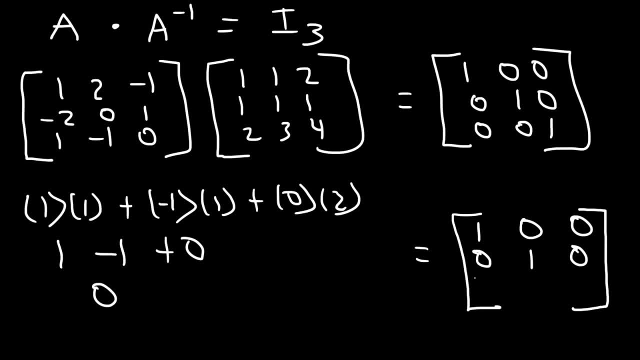 So it's 1 minus 1 plus 0, which is going to be 0.. Next is going to be row 3 and then column 2.. So this takes some time. I mean it's pretty laborious, but that's how you can confirm it. 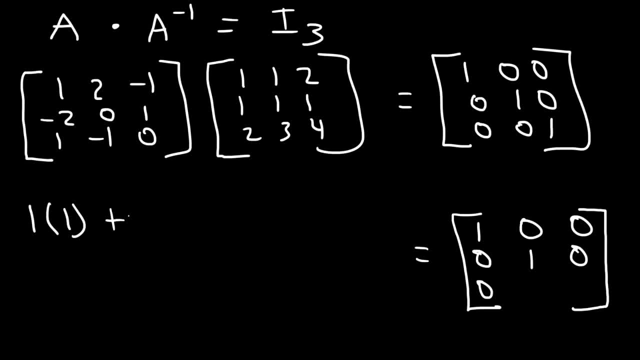 So it's going to be 1 times 1 plus negative, 1 times 1, and then 0 times 3.. So this is 1 minus 1 plus 0, which is 0.. And finally, the last one. 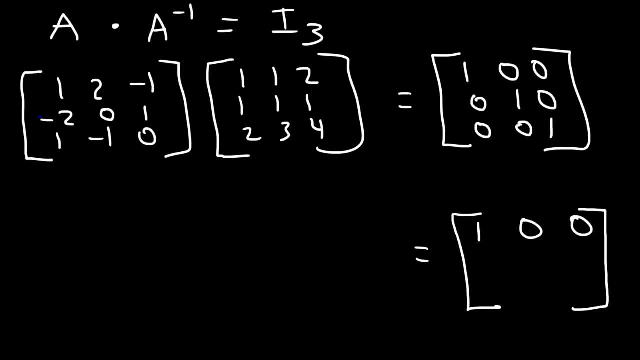 now let's move on to row 2. now let's multiply it by column 1, so it's going to be negative 2 times 1 plus 0 times 1 plus 1 times 2. so this is negative 2 plus 0 plus 2. negative 2 plus 2 is 0. 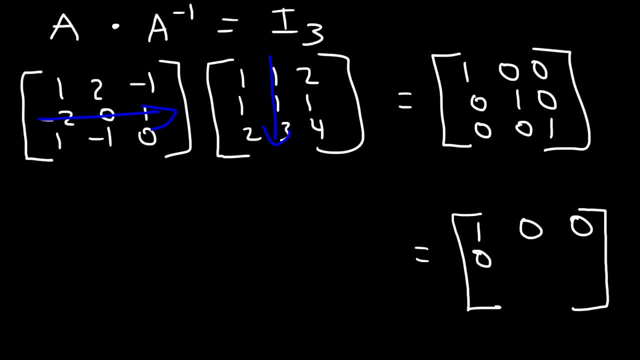 now let's take row 2 and multiply it by column 2, so it's going to be negative 2 times 1 plus 0 times 1 plus 1 times 3, so that's negative 2 plus 0 plus 3 negative. 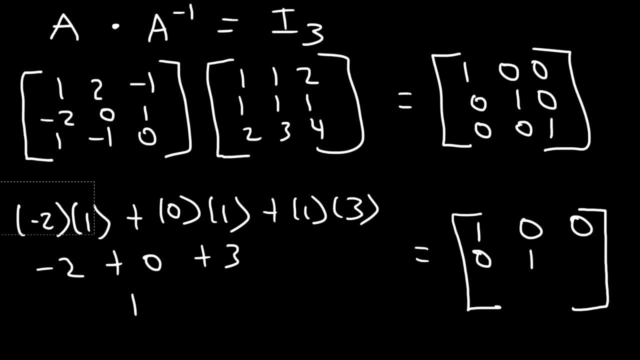 2 plus 3 is 1. now let's multiply row 2 by column 3, so negative 2 times 2 plus 0 times 1 plus 1 times 4. so this is going to be negative 4 plus 0 plus 4, which adds up to 0. 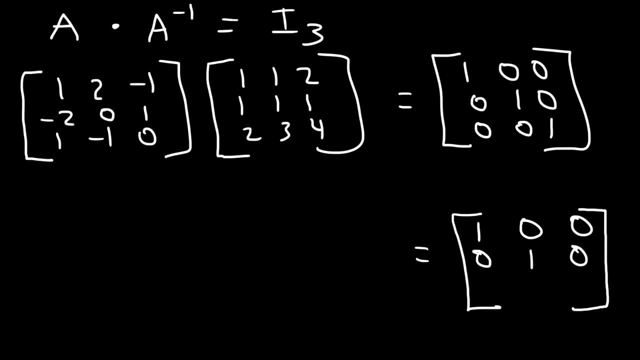 now row 3 times column 1, let's try that. so it's going to be 1 times 1 plus negative 1 times 1 plus 0 times 2, so it's 1 minus 1 plus 0, which is going to be 0. 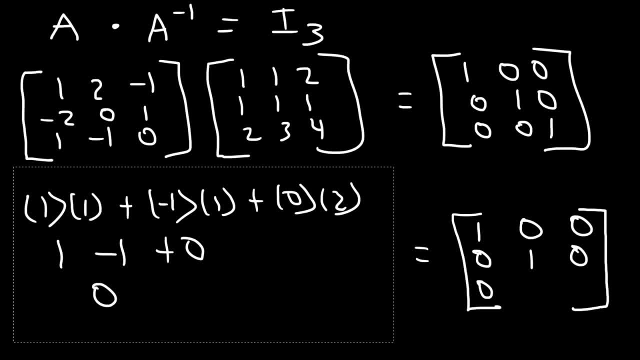 next is going to be row 3 and then column 2, so this takes some time. I mean, it's pretty laborious, but that's how you can confirm it. so it's going to be 1 times 1 plus negative, 1 times 1 and then 0 times 3, so this is 1 minus 1 plus 0, which is 0, and finally. 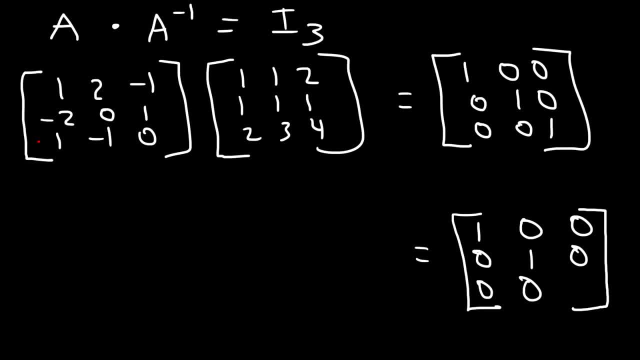 Here it's going to be row 3 times column 3. So that's going to be 1 times 2 plus negative, 1 times 1 plus 0 times 4.. So it's 2 minus 1 plus 0.. 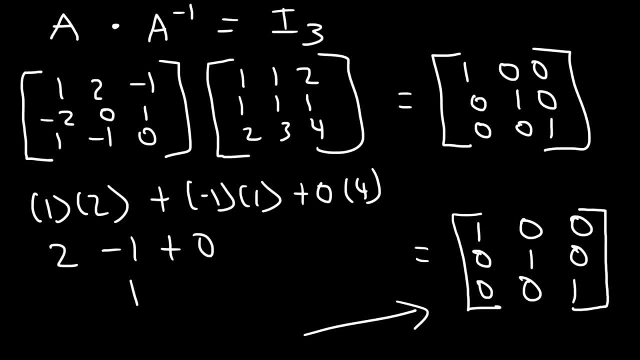 2 minus 1 is 1.. And so we do get the identity matrix. So that tells us that this is indeed the inverse. So now you know how to find the inverse of a 3 by 3 matrix. Thanks for watching. 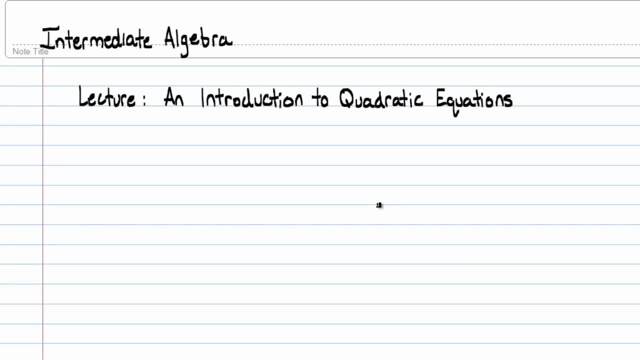 Hello, my name is Roy Simpson. I'm an instructor of mathematics at Cosumnes River College in Sacramento, California. This is a first in a series of lectures on quadratic equations and how to solve quadratic equations and how to solve quadratic models and build quadratic models. This is essentially your first foray into a really detailed exploration into parabolas and quadratics, things that are not linear in mathematics. And in the first attempt here, we're going to go ahead and define what a quadratic equation is. And then from there, we'll talk about what a quadratic equation, maybe the different forms it takes and how to solve those different forms. 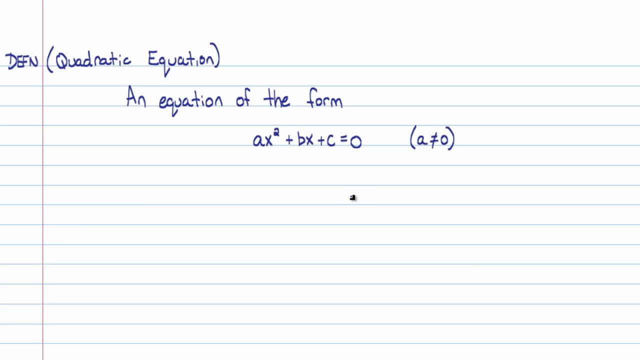 Now, the official definition of a quadratic equation is an equation of the form ax squared plus bx plus c is equal to zero, where a is non-zero. If a is going to be equal to zero, then a is going to be equal to zero. If a is going to be equal to zero, then a is going to be equal to zero. The reason why we say a cannot be zero is that if it is, then it's just bx plus c is equal to zero. And that's actually a linear equation. 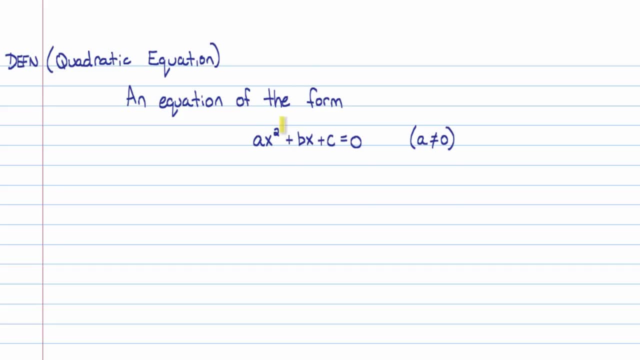 So you'll see the difference between a linear equation and a quadratic is this power of two placed on the exponent of your variable. So that's essentially how you're going to tell that you have a quadratic equation is when you have an equation, first of all. And that the power. On your lead term is two. 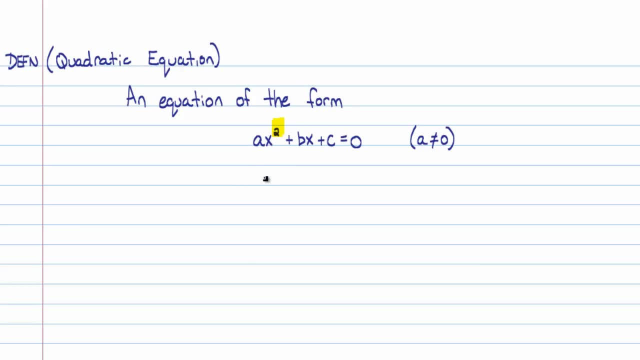 And then there's all these different types and forms of quadratic equations. And maybe I should show you a few of them here. Something like if you have ax squared plus bx is equal to c. That's also a quadratic equation. Ax squared is equal to c.